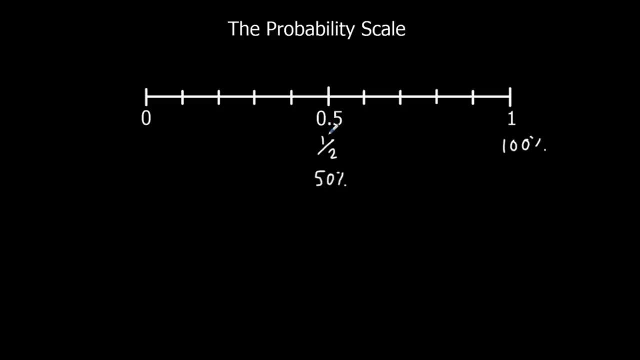 if it's in the middle, it's got a 50% chance- 1 in 2 chance- of happening. So this is what the probability scale is like, and any probabilities always have to be out of one whole Okay. so here we've got a. 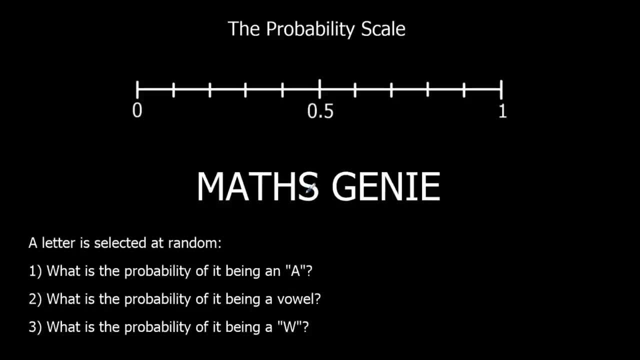 question. It's got the letters here of Maths Genie and it says: a letter is selected at random. What's the probability of getting an A? Well, if you have a look here, you can see there's only 1 A out of 10 letters, so it's 1 out of 10.. So if I'm going to mark, 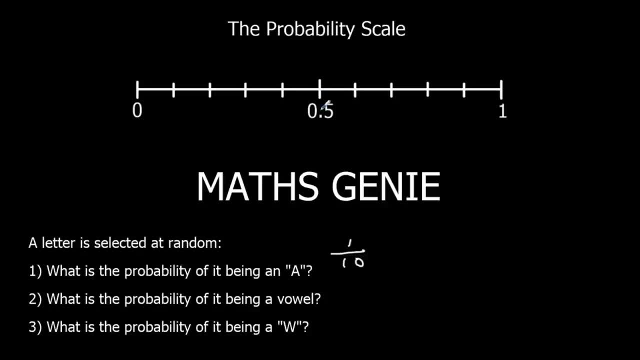 this on the probability scale up here this is 50%, That's 5 out of 10, 4 out of 10, 3 out of 10.. This is 1 out of 10 over here. So that's the probability of getting an A. What's the? 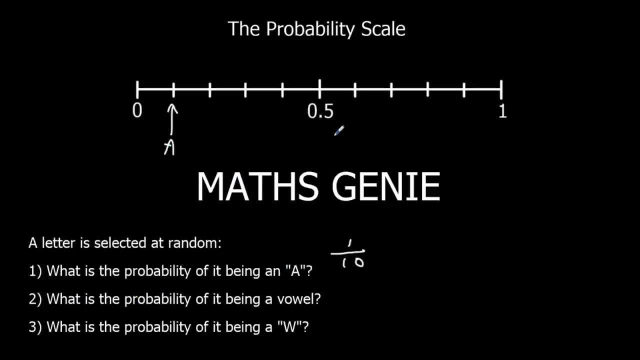 probability of getting a vowel. So there's 1,, 2,, 3, 4.. 4 vowels out of 10 letters, so it's 4 out of 10.. 4 out of 10 is here, So 4 out of 10, that's the probability of getting. 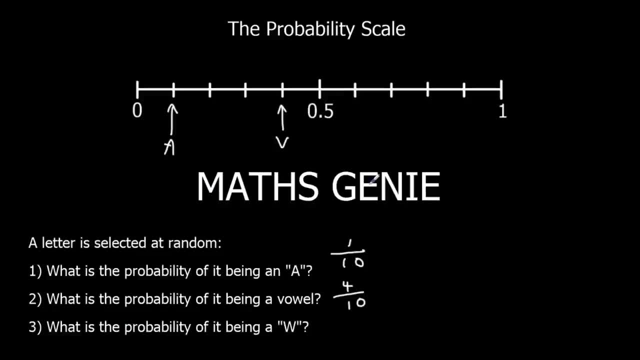 a vowel, And what's the probability of getting a W? Well, there's no W's there, So it's zero. There's no chance, zero out of 10.. So probability to get a W is there. Okay, have a go at this one to see if you can answer these questions and mark them. 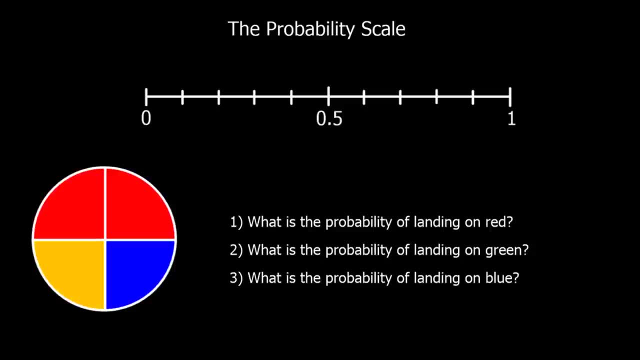 on the scale, Okay, the probability of getting a red on this spinner. well, there's 2 reds out of four, so it's 2 out of four And that's a 50% chance: 0.5.. So probability of getting. 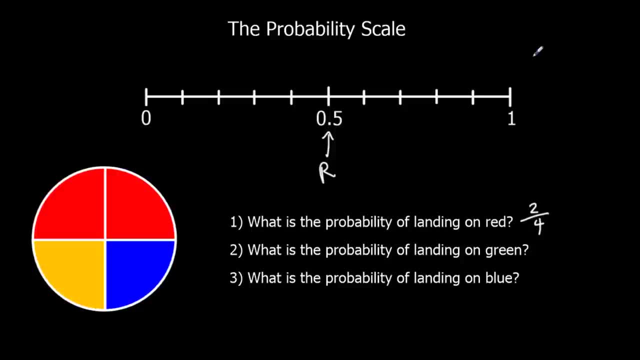 a red is 0.5 out of 10.. There we go, we've done it. This is 1, 2, 3, 4.. That's 1 out aquí, zero point five. what's the probability to get a green? there are no greens, so